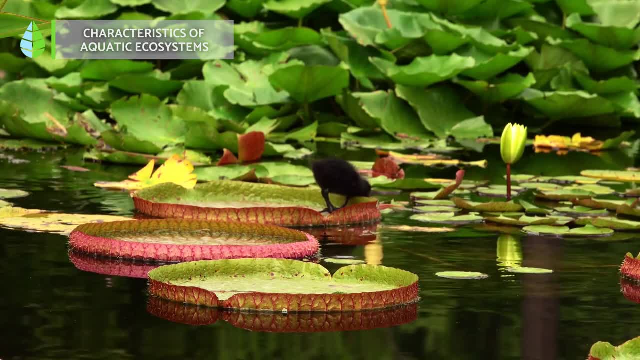 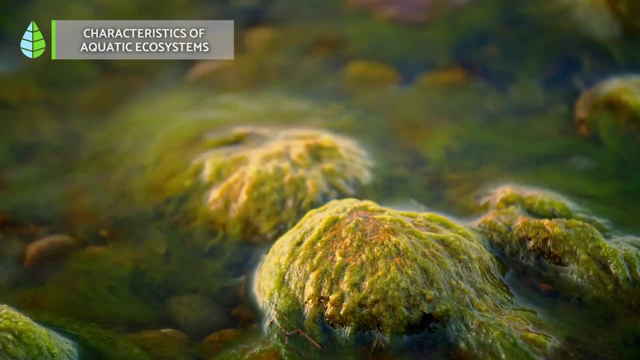 both those that can only live in water and those that inhabit both water and land or sky. They are one of the richest ecosystems in the world, as they have a great biodiversity. Its flora is made up of algae and aquatic plants. They have vital functions for the planet. 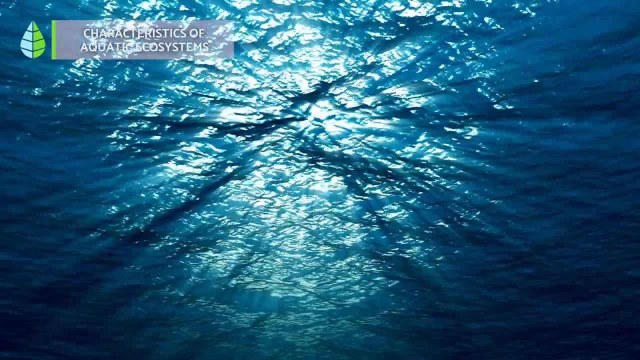 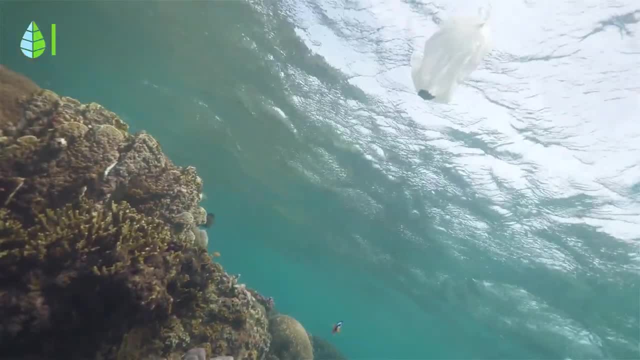 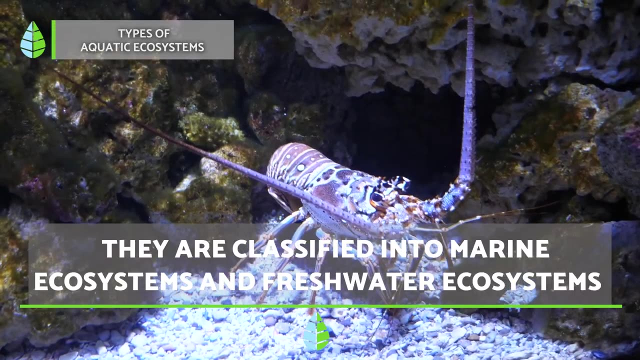 such as helping to regulate the water cycle throughout the planet, shaping the environment. They are an environment of a great variety of species that otherwise would not exist and also acts as a filter for pollution. Types of Aquatic Ecosystems: These ecosystems can be divided into two large groups: marine and freshwater ecosystems. 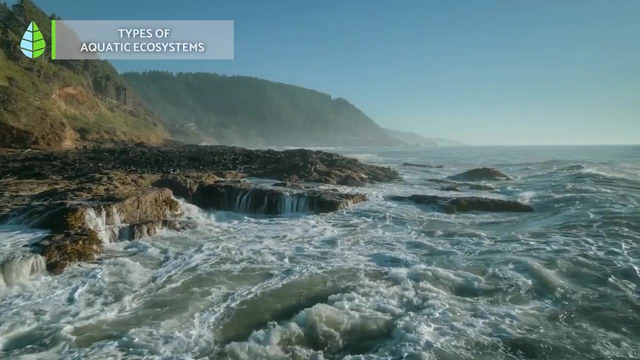 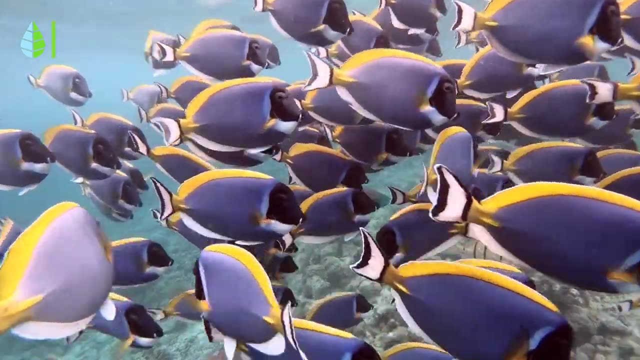 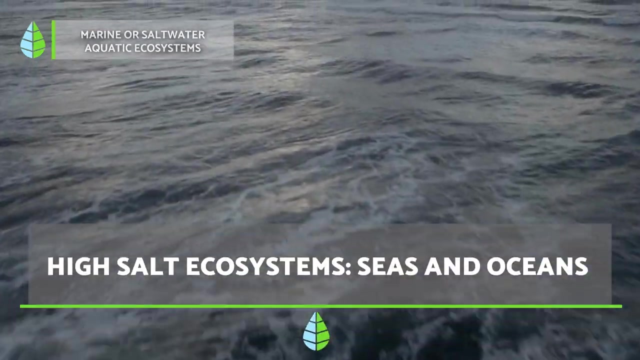 In addition, these types of ecosystems can also be classified into lotic ecosystems, if the water is in motion, or lentic ecosystems, if it is still, or with little movement. Marine or Saltwater Aquatic Ecosystems. Marine ecosystems are those with a high level of salt found in areas between continents and 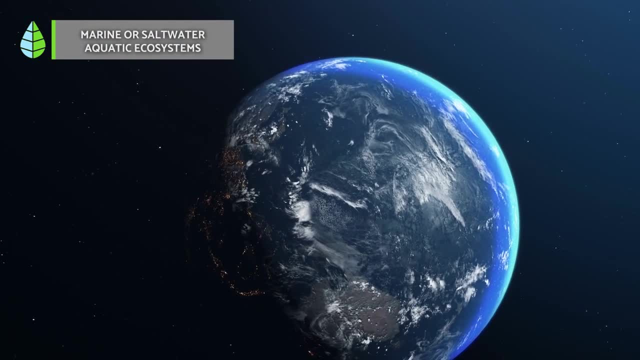 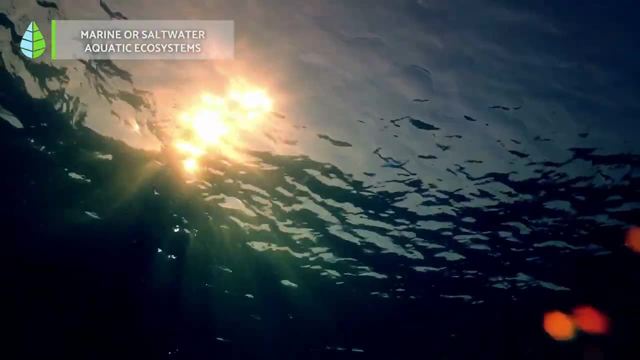 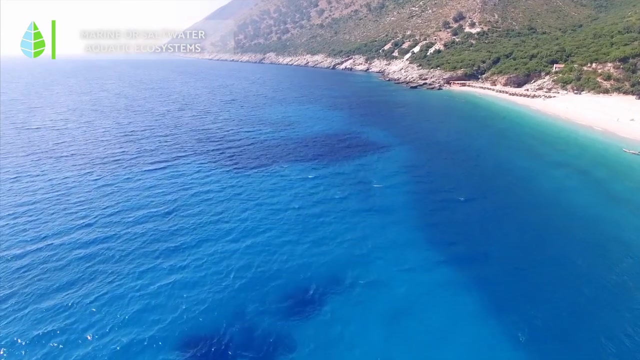 surrounding islands. These represent 70% of the earth's surface and 99% of its volume. We're talking about salty waters, such as seas and oceans At abysmal distances. most of the ecosystems are unknown. Still, it can be argued that coastal areas are more populated. 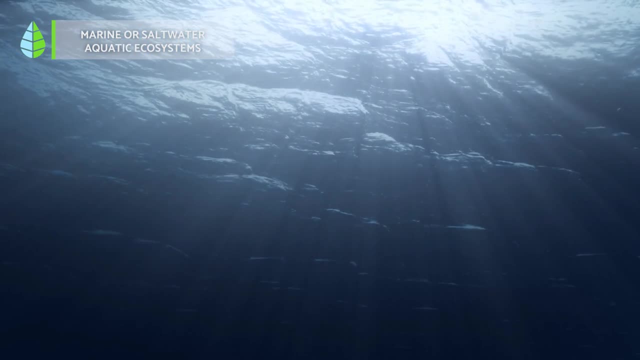 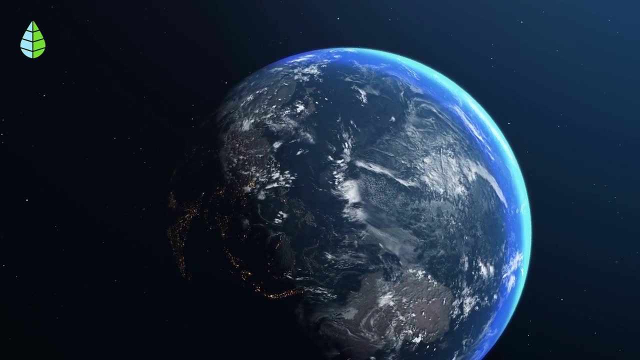 than the inhospitable seabed. This, in large part, is because the food chain begins with plankton and it needs sunlight to grow. Before we continue, let's put you to the test Of all the water on the planet. what percentage is freshwater? 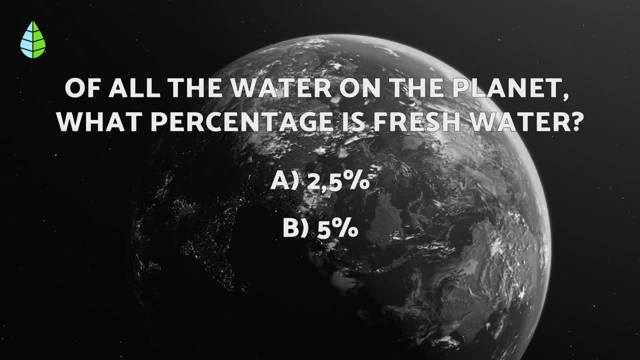 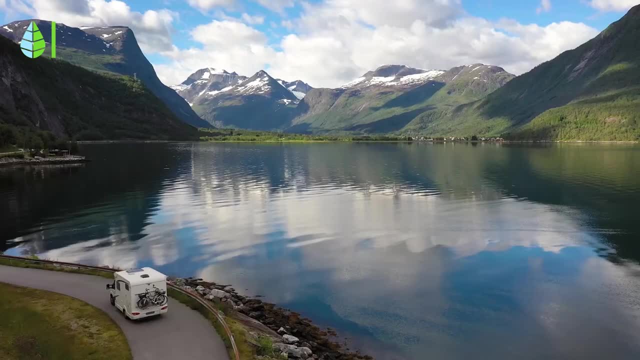 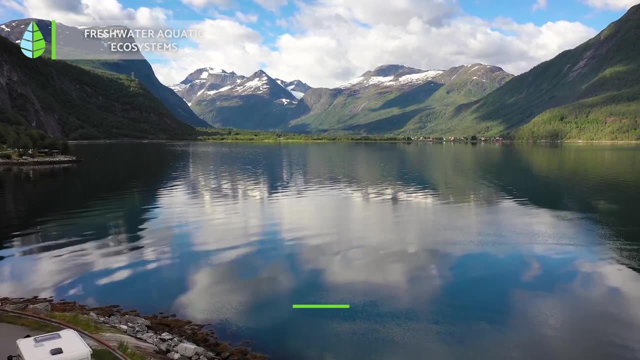 A 2.5%, B 5% Or C 7.5%. Think about it, because at the end of the video you'll find out if you're right. Freshwater- Aquatic Ecosystems. Freshwater ecosystems are found in places where we find waters that are low in salt. 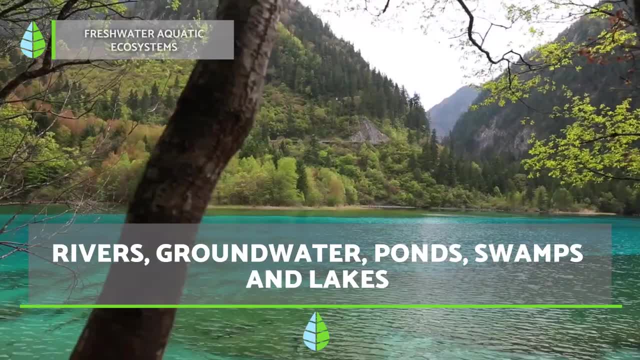 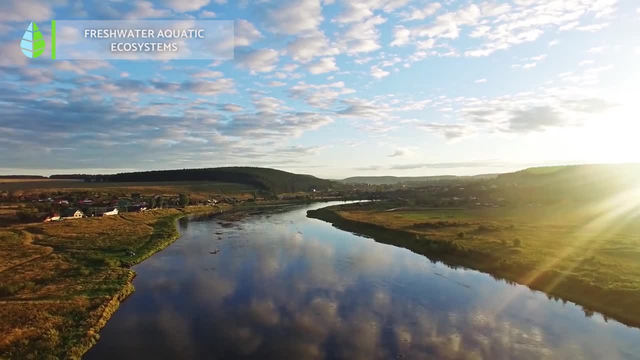 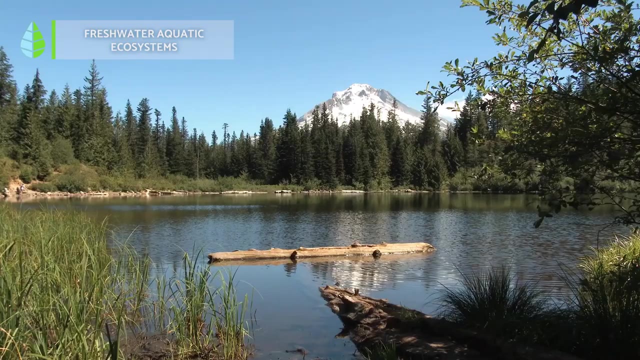 such as rivers, groundwaters, ponds, swamps and lakes. Unlike the marine ecosystem, its depth and diversity of fauna and flora is less, although it's still very rich. Various factors, such as the weather and the relief determine the characteristics of the habitat, For example, the flora and fauna of a shallow. 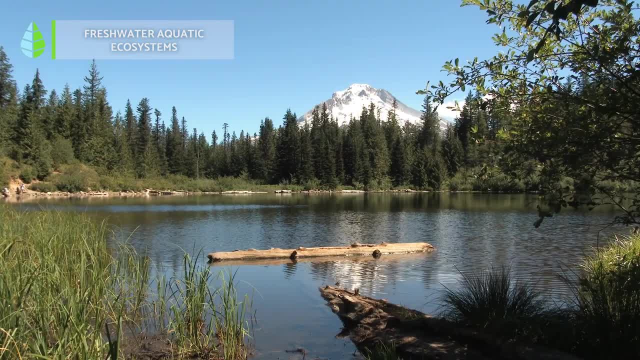 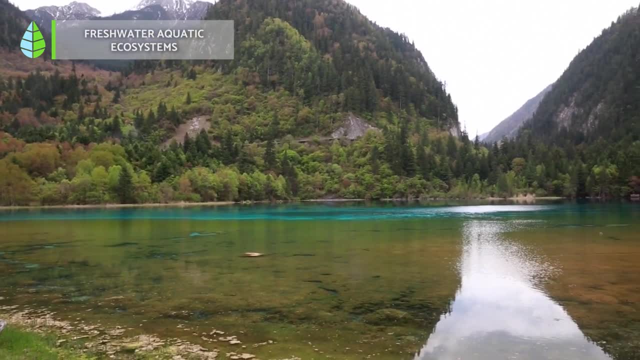 lake in a northern mountain will be very different and incompatible with that of a shallow, warm-water lake in a tropical climate zone. The ideal conditions are created in each ecosystem for these lifeforms to flourish. Flora of Aquatic Ecosystems. Flora of Aquatic Ecosystems. Flora of aquatic.